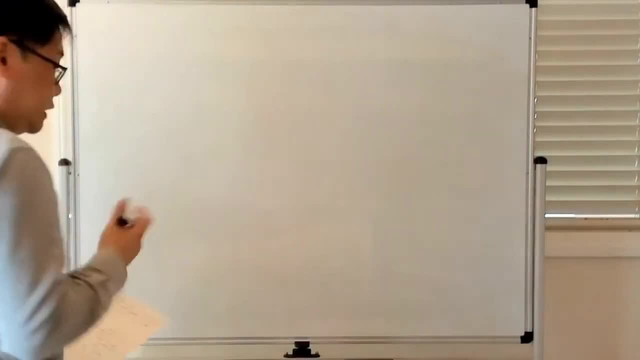 Okay, so now I'm going to talk about a particular topological invariant called the Euler characteristic, And the Euler characteristic is going to turn out to be related to the number of holes, if you will. So, if you recall, it's like we talk. 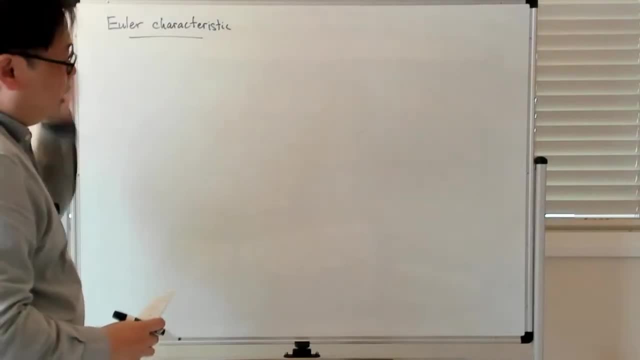 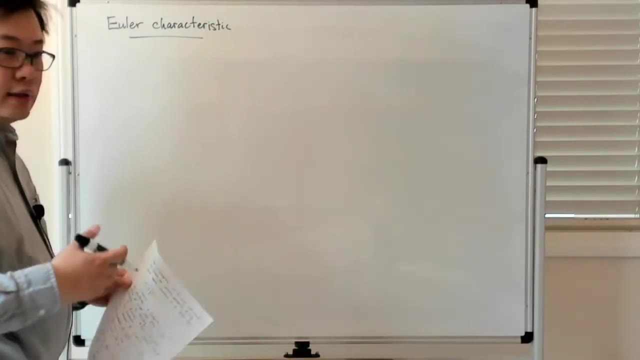 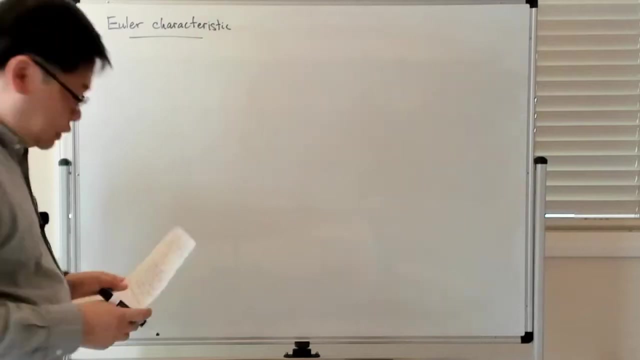 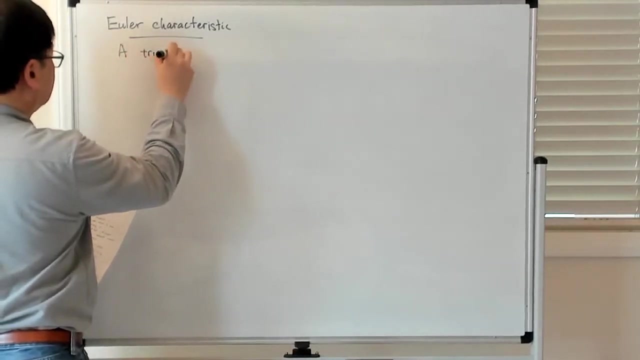 about a classification of compact two manifolds without boundary, and we had this idea that you know you could obtain this by either looking at spheres as well as connected sums of either projective planes or connected sums of. you know, it's like the torus, okay, So all right. so you know that a triangulation, 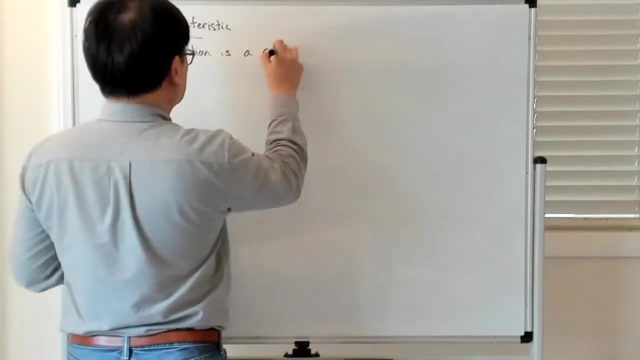 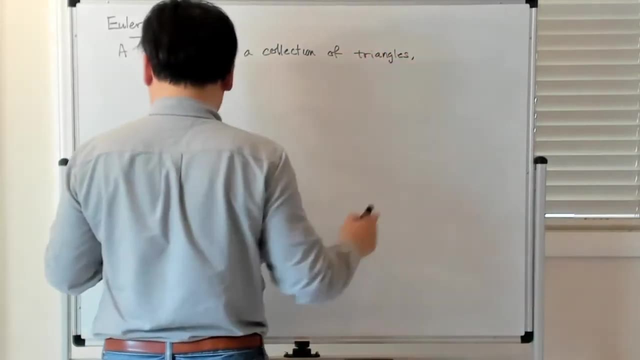 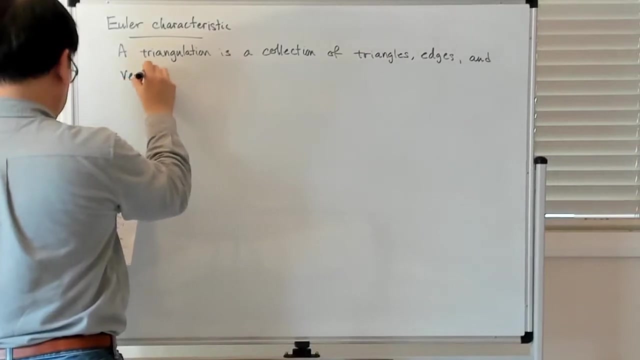 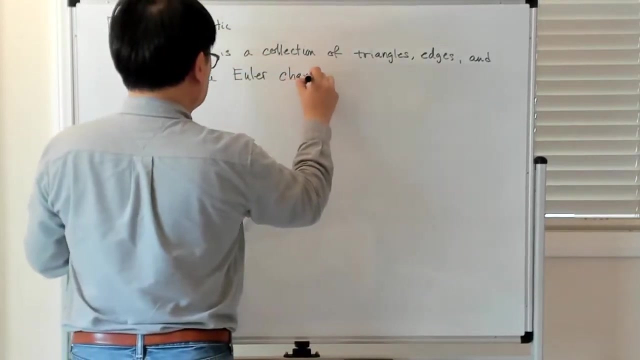 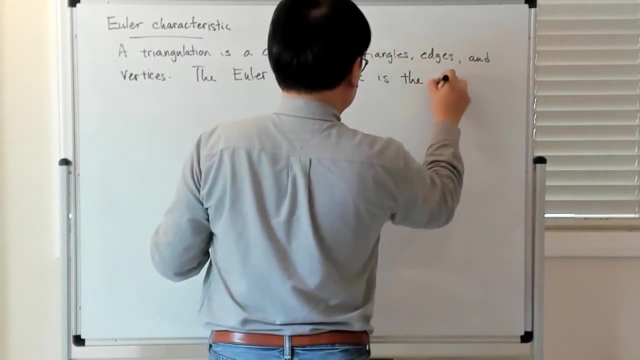 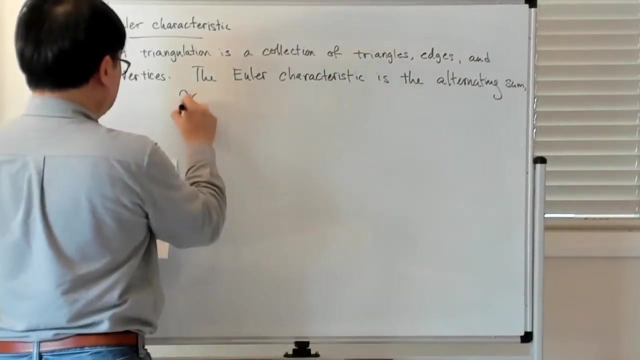 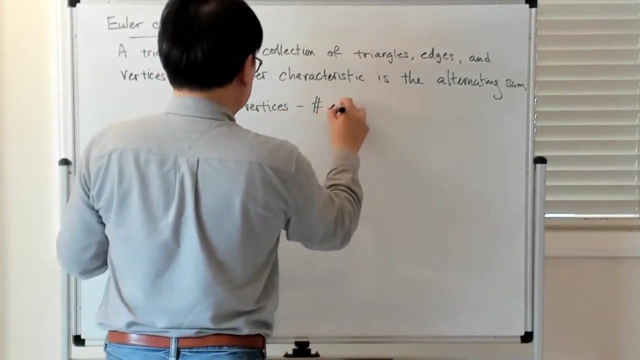 is a collection of triangles, edges and vertices. All right. and then the Euler characteristic is the alternating sum given by the followers. okay, So because c is equal to the number of vertices minus the number of vertices, So c is equal to the number of vertices minus the number of edges, plus the number of triangles. 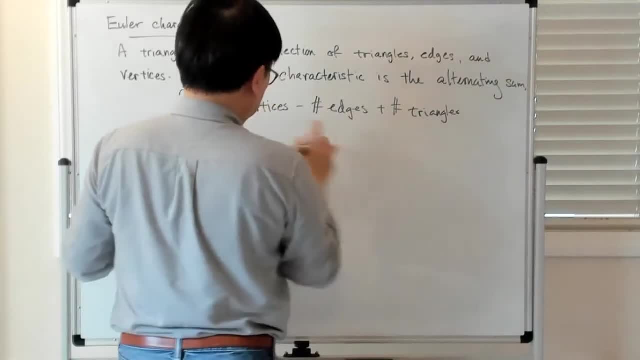 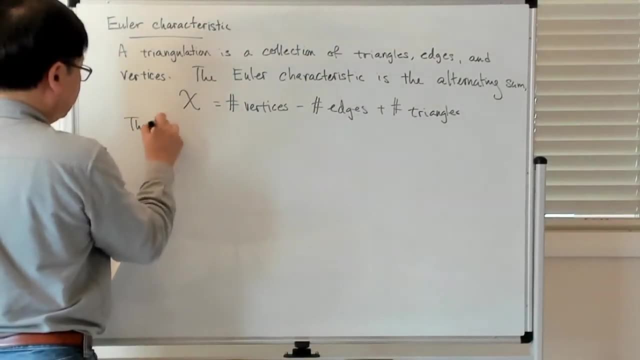 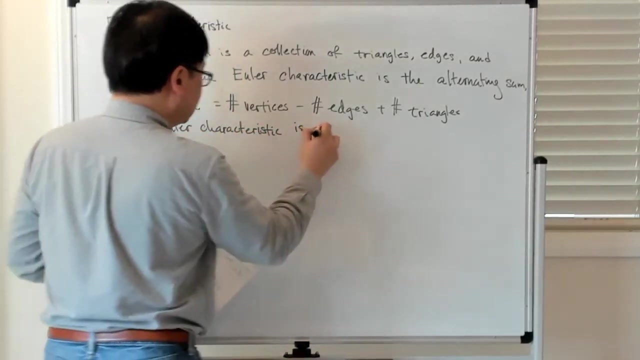 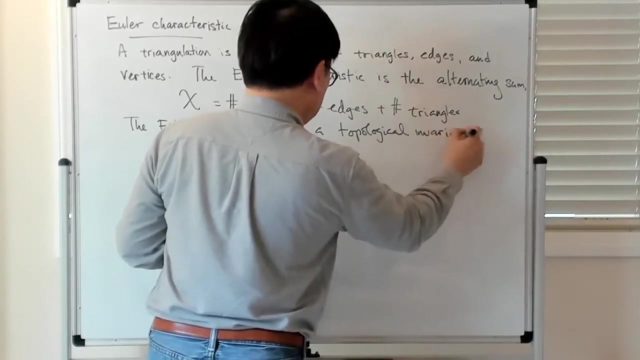 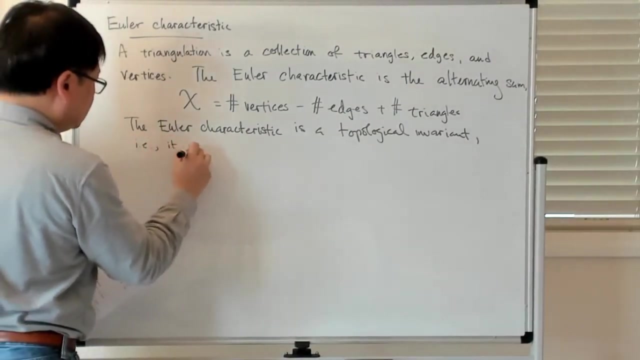 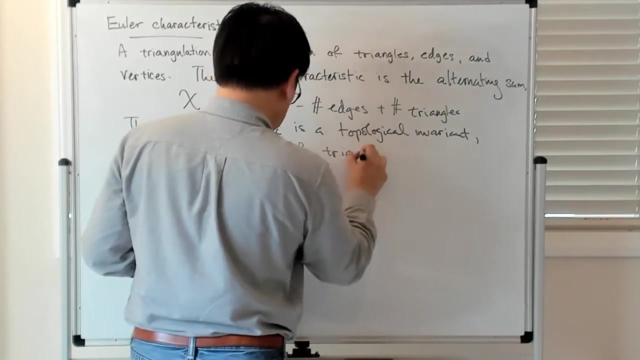 All right, and you can see that. you know, the ordering is in terms of increasing dimension. okay, So the Euler characteristic is a topological invariant, Okay, Okay, And as a consequence, it is independent of triangulation. 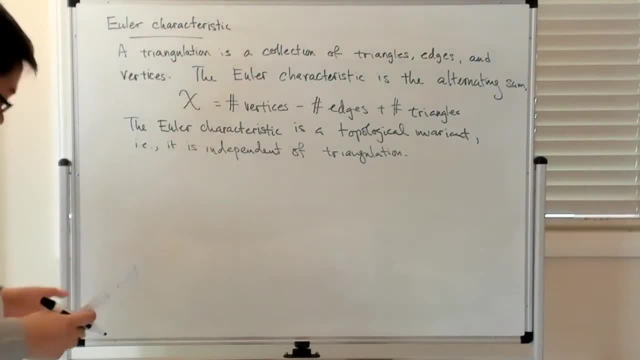 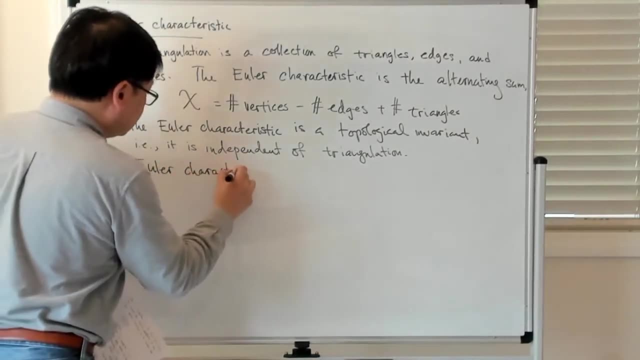 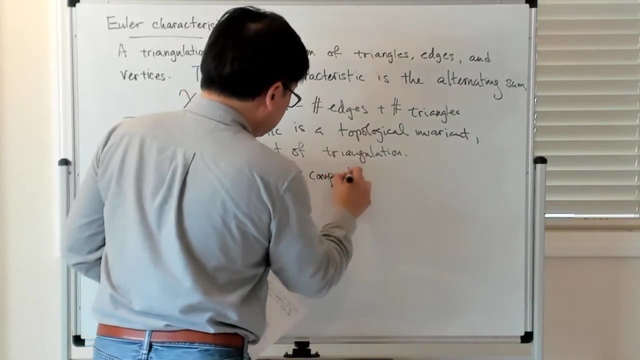 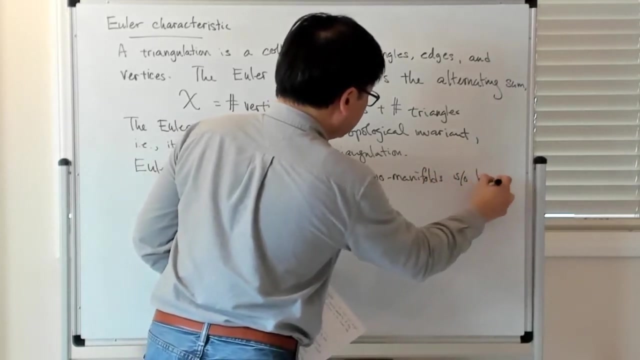 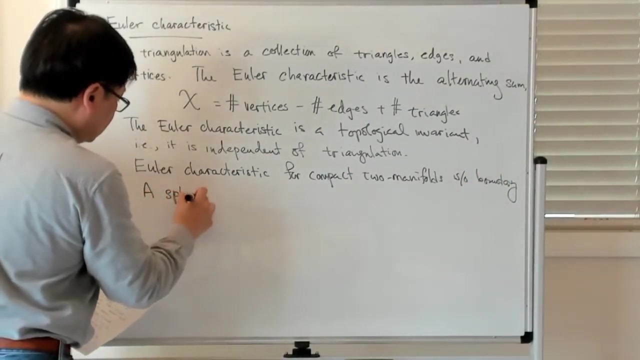 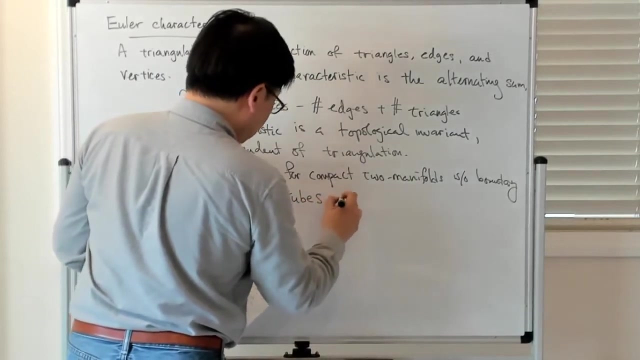 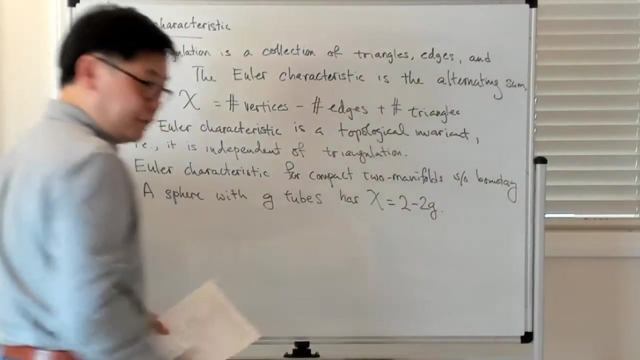 So now we can see something about the Euler characteristic for these compact two manifolds which he had classified earlier without boundary. So a sphere with g-tubes has Euler characteristic which is 2 minus 2g. So g is oftentimes referred to as the genus which has to do. 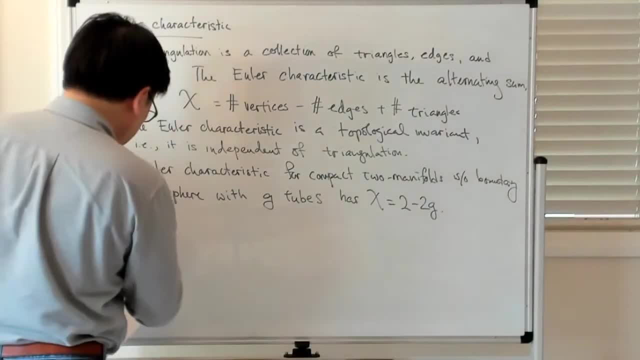 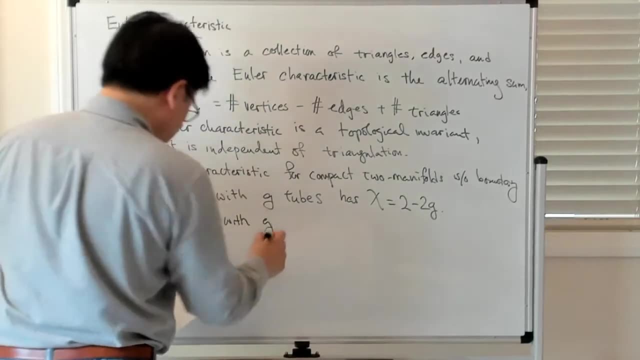 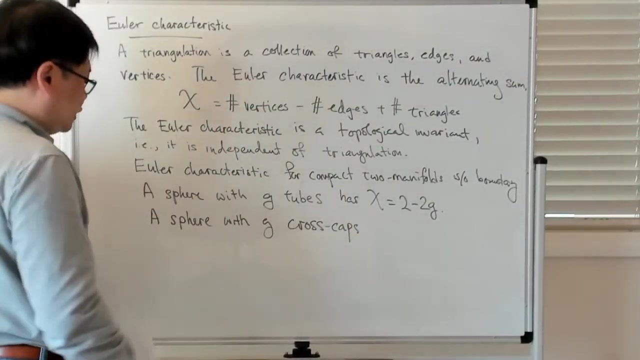 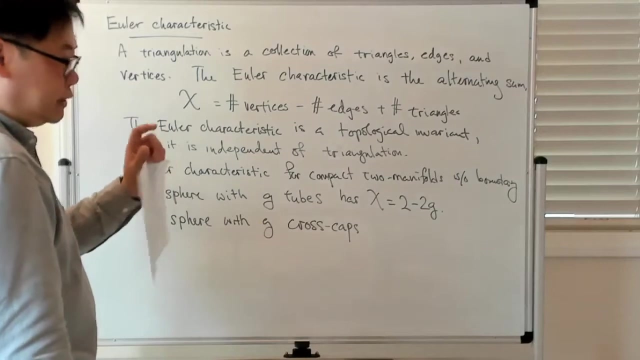 intuitively with the number of holes you have in the manifold And a sphere with g cross caps. So I should say what's happening, of course, is that if you have these, it's like a sphere with g-tubes. you're basically taking the sphere and you're 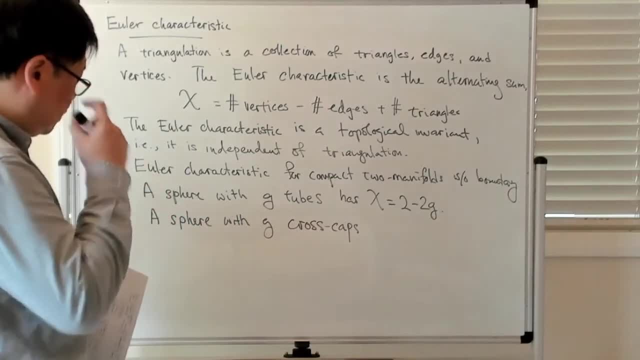 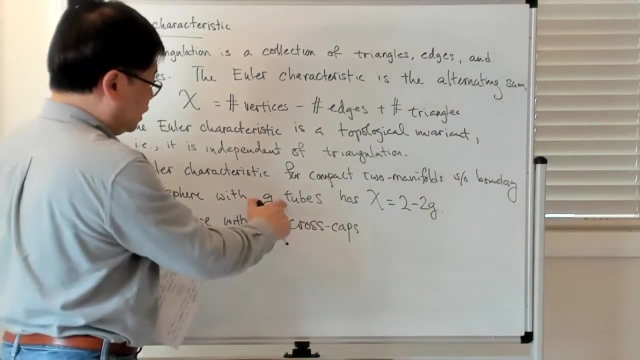 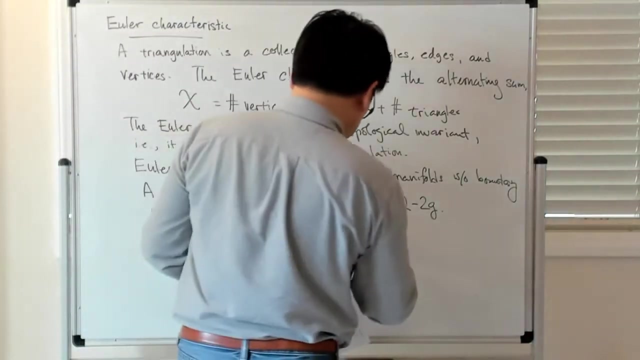 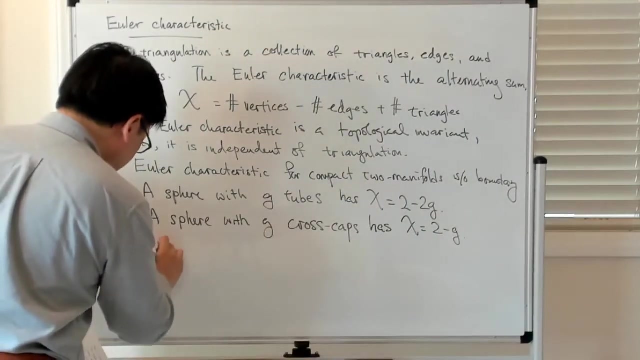 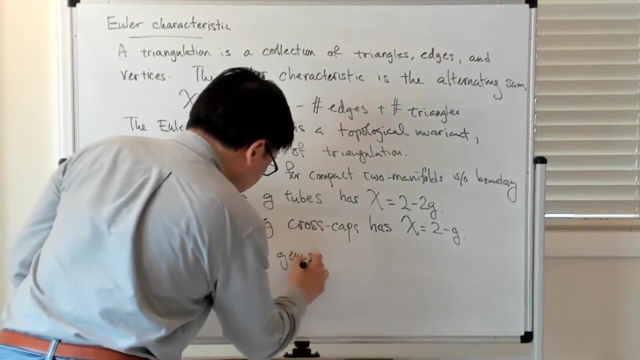 looking at the, in some sense the connected sum of the sphere with either the torus or the projective plane. So that's where the g is coming from. So this has Euler characteristic 2 minus g. So g here denotes the genus. 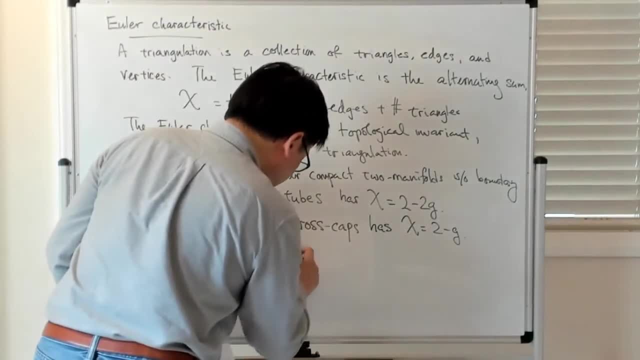 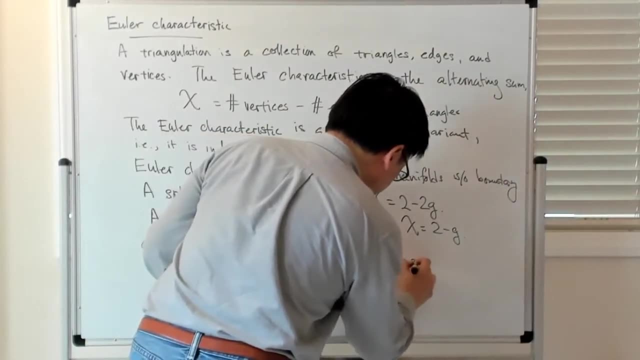 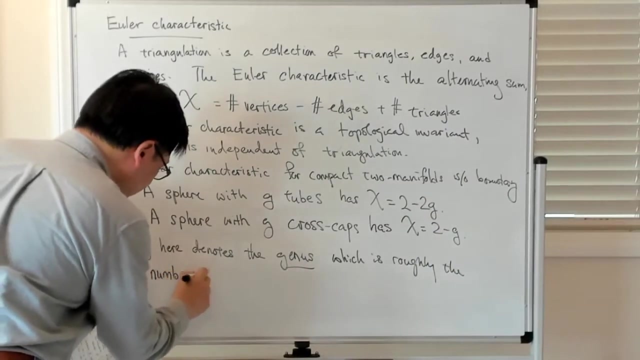 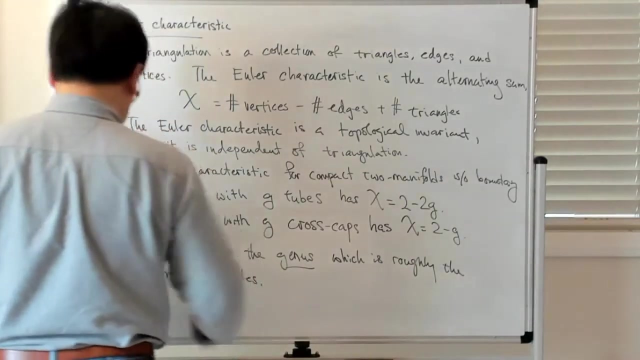 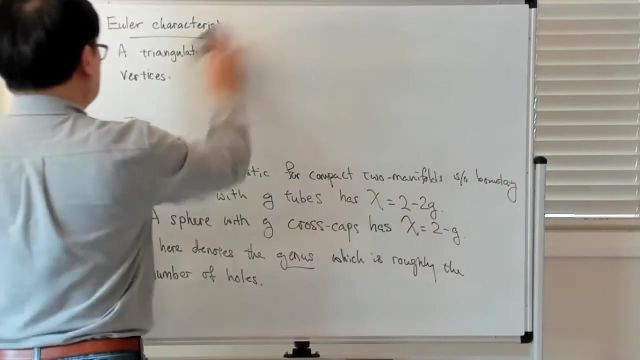 g-e-n-u-s, which is roughly the number of holes. Okay, All right. So let's look at what the genus is and the Euler characteristic is for some of these compact two manifolds without boundary. Okay, so I'm going to denote by n. 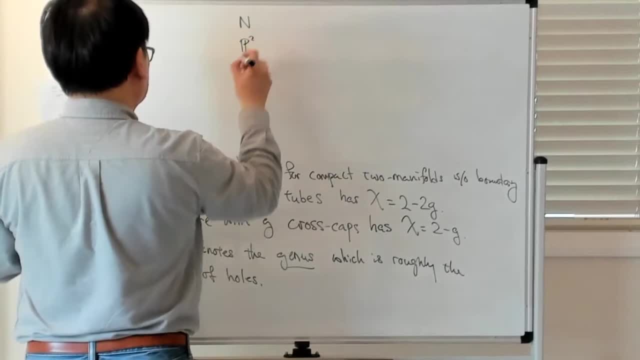 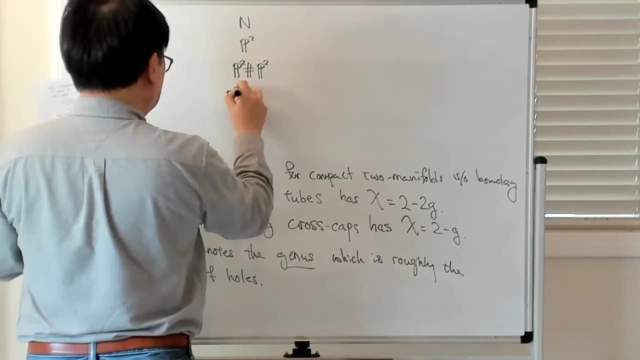 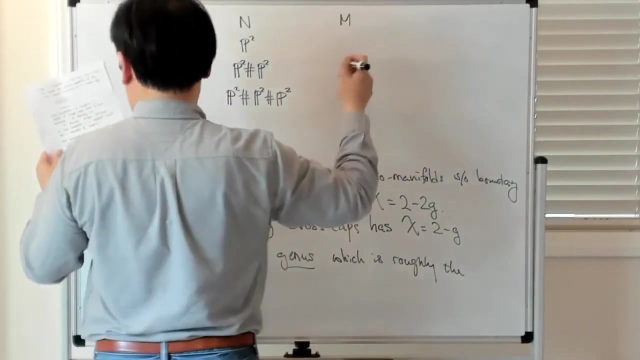 it's like the non-orientable things, like the projective plane, sort of the connected sum of two copies of the projective plane and sort of connected sum of three copies of the projective plane. And then m denotes the orientable things. 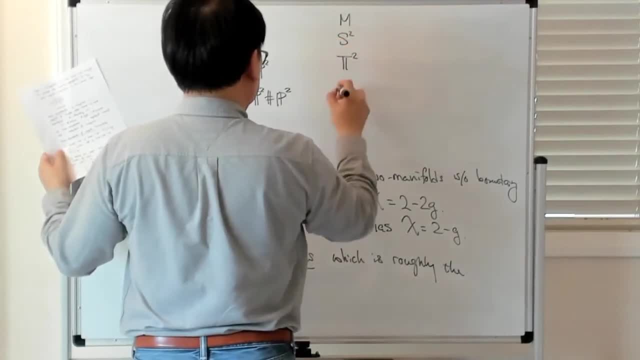 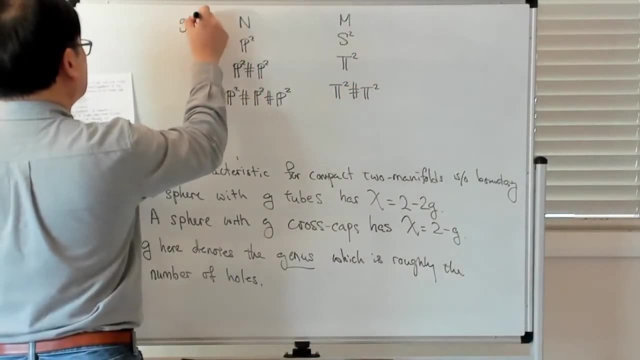 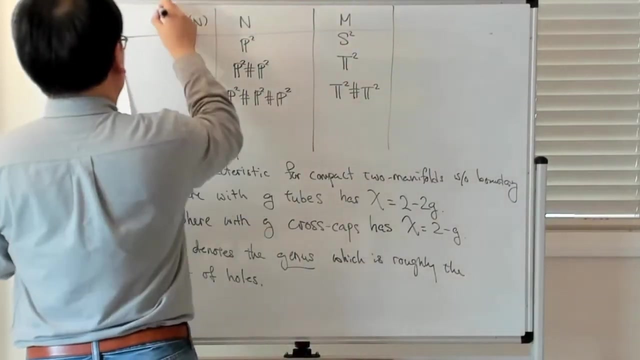 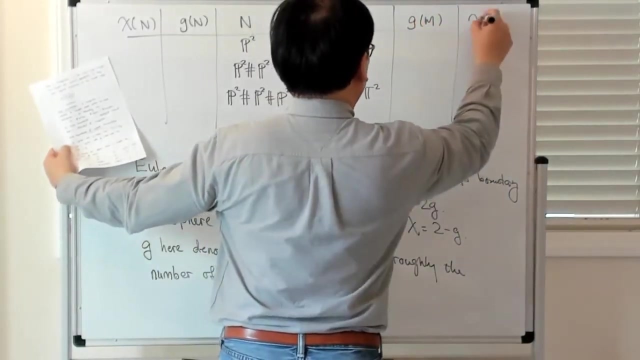 like the two sphere, two torus, the two torus connected with itself, Okay. And then there's the genus: Okay, And the Euler characteristic, and the genus and the Euler characteristic, Okay. So the sphere obviously has genus zero. 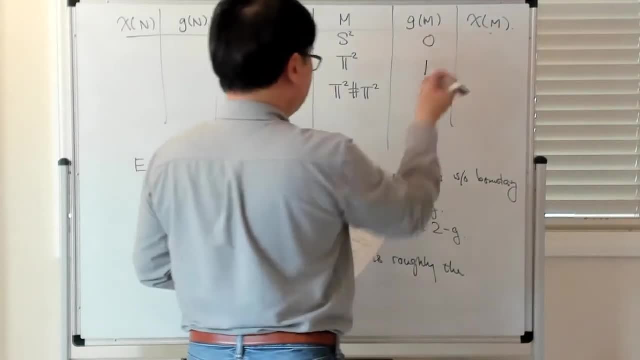 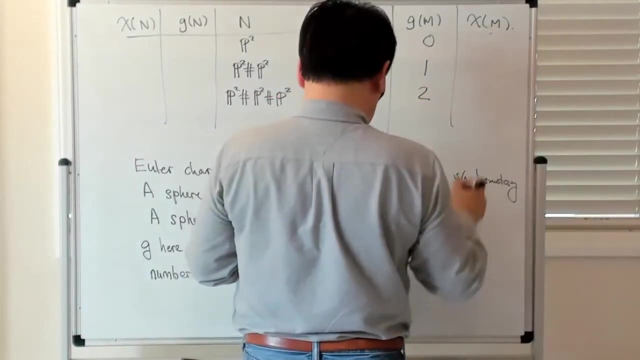 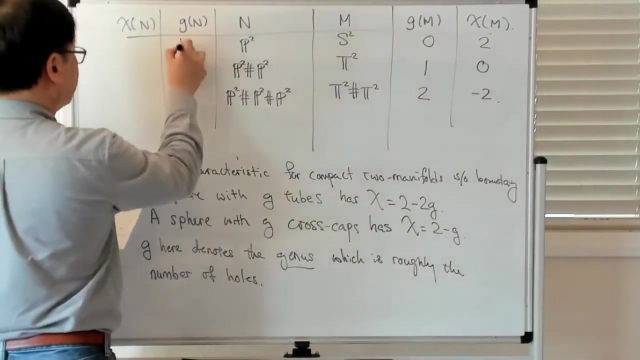 has no holes Right. Then the torus has one, and then connected sum of the two tories have genus two. Okay, The Euler characteristic here is two zero and minus one. And then here your genus one, two and three.